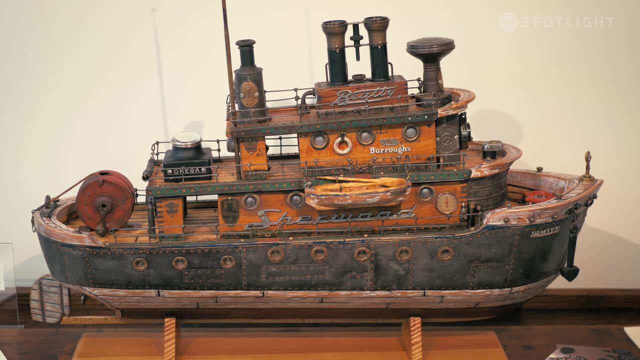 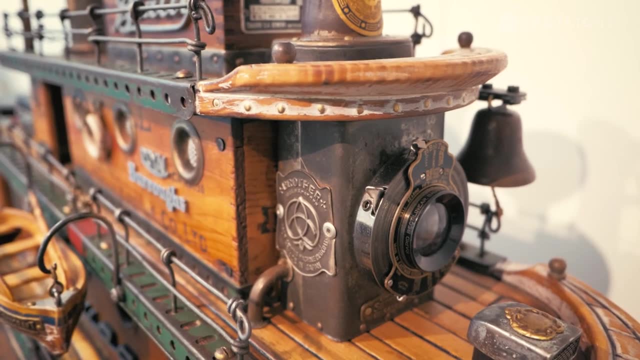 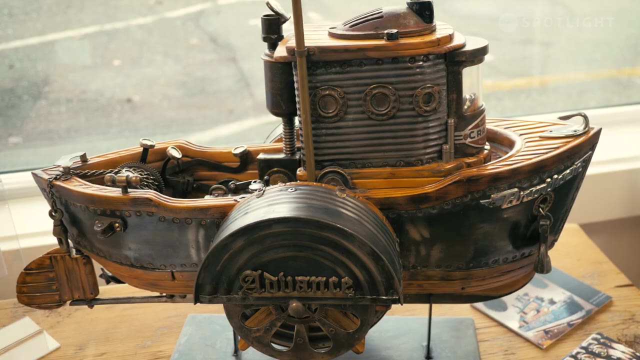 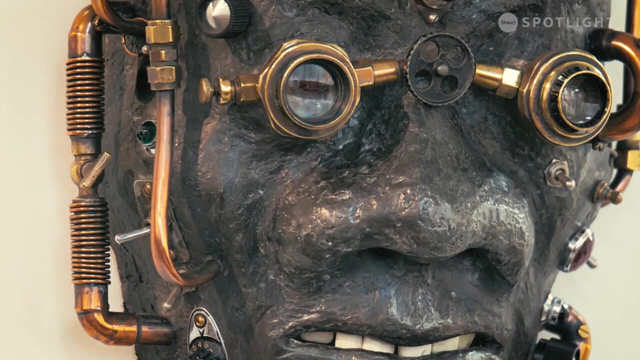 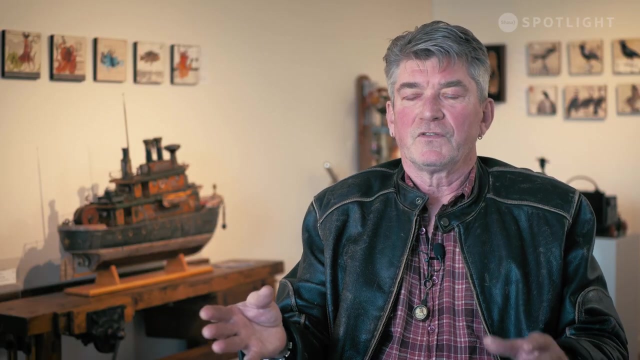 It was just how I sculpted and how I assembled things. But I found out later that it had a title and apparently that I was making nice things with it, And that was steampunk. What's put me off in this direction is I've basically always been a recycler. 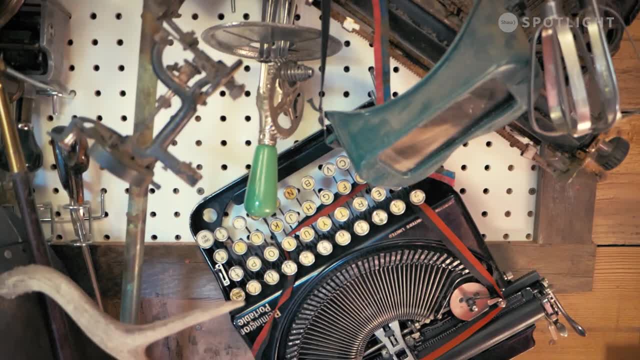 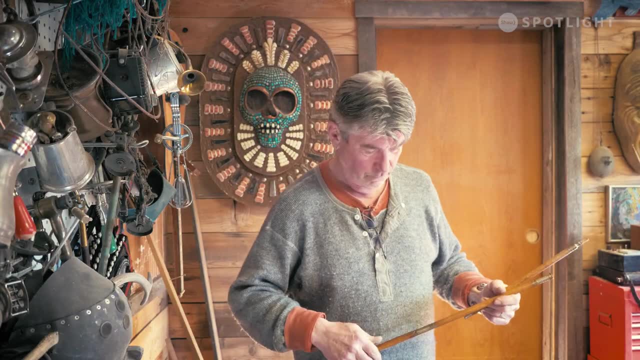 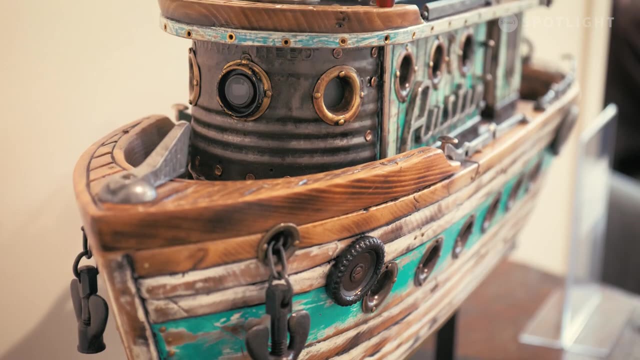 I like to repurpose things and see them in a different way than they were actually Maybe purposed for. I spent a lot of time down at the harbour. I love boats. I don't own a boat, but I love basically everything about boats. 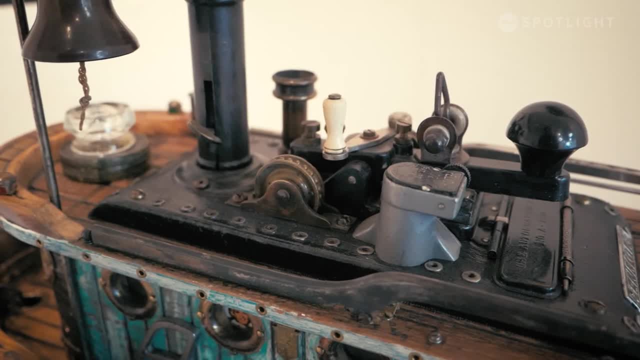 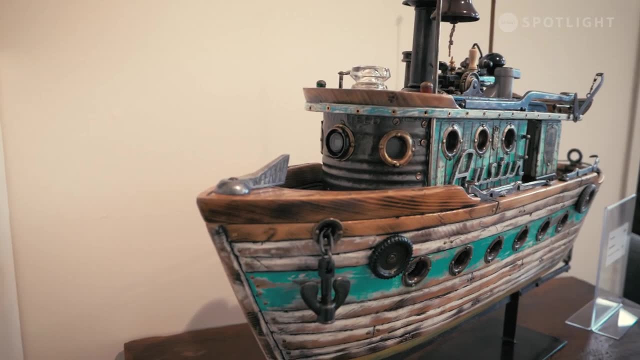 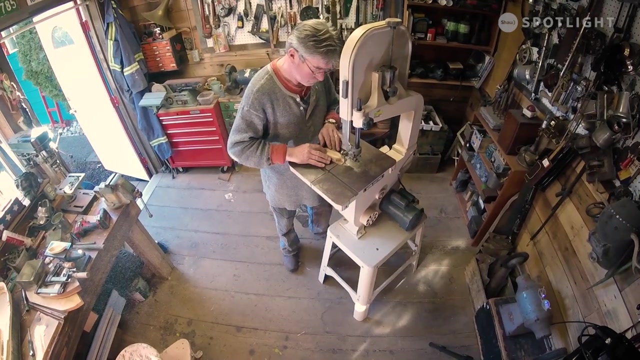 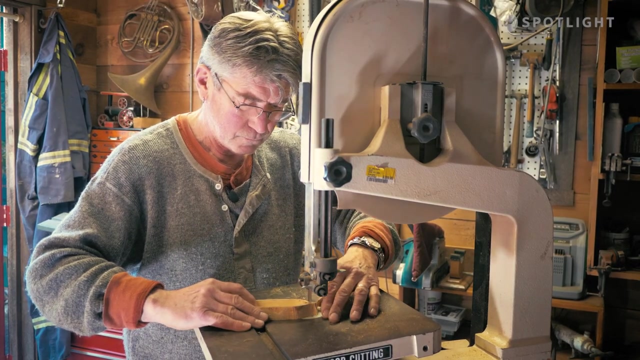 So I started to make these boats. Although they're not planned, measured, they're planned in my mind and I know where I need to go. So they're not scale models, They're just sculptures. I kind of get lost when I go into my shed and when I start actually working a piece. 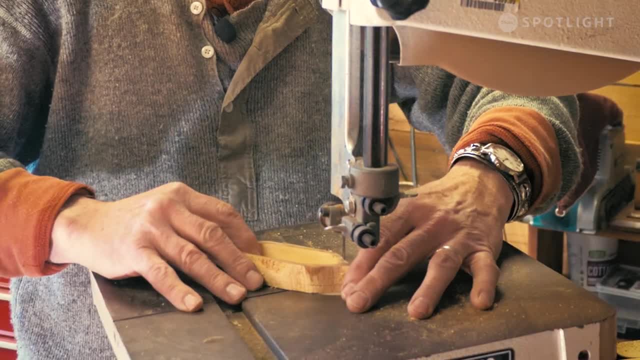 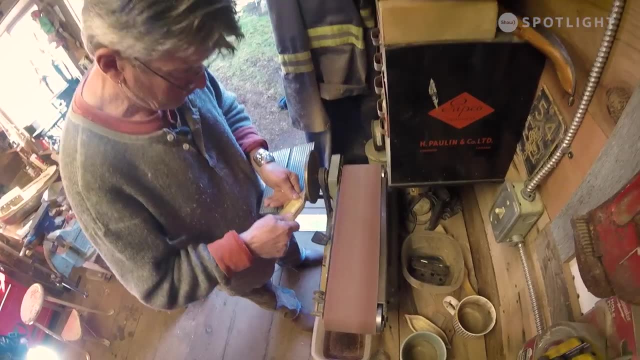 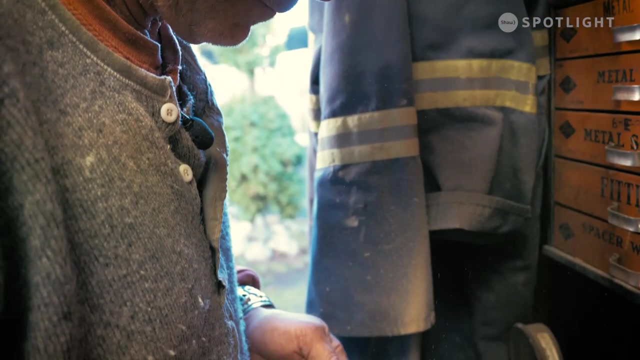 because it's not uncommon at all for me to come out from my work 14 hours later. I can go in in the morning and I can come out at 10, 11 o'clock at night time, And that's something that it's not a labour to me. 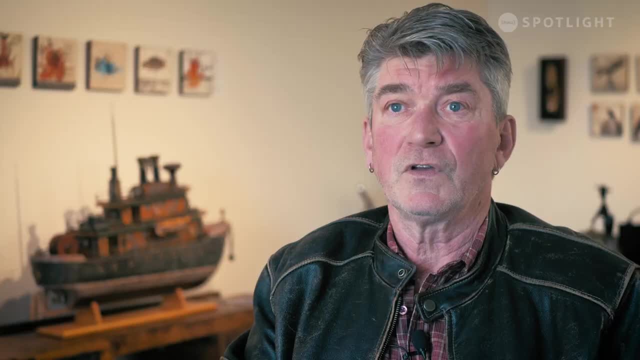 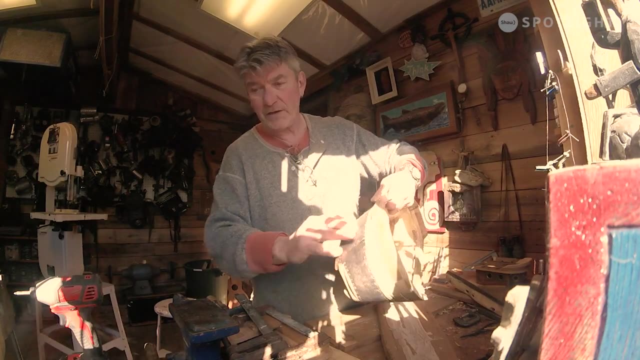 I don't feel like I'm being tortured or anything. I'm just lost in time and I'm in my zone, So it's a really for me, it's a really good place to be. The metal on the side here, this flat stock, is actually cake tins- square wedding cake. 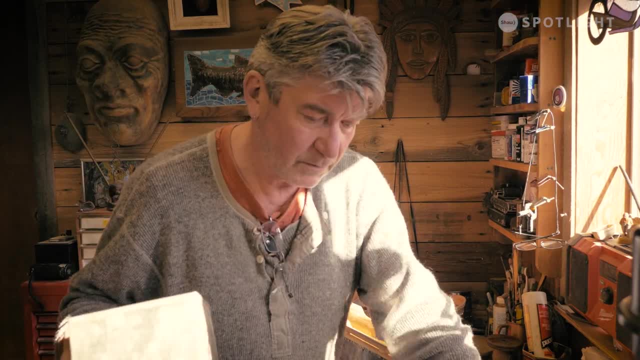 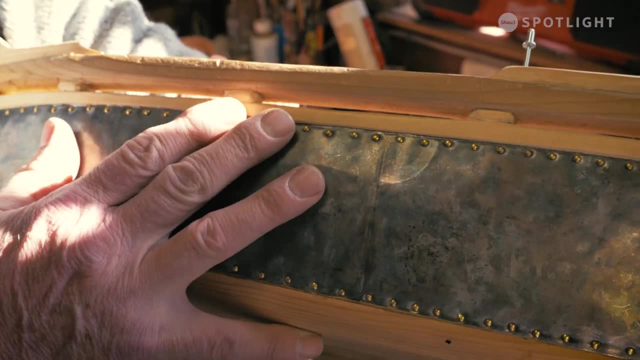 pans with the pop out bottom. But because it's an old metal, I get a really nice colour when I burn it. I hammer it and I burn it. I get a great texture from it. It's really nice, I get a great texture from it. 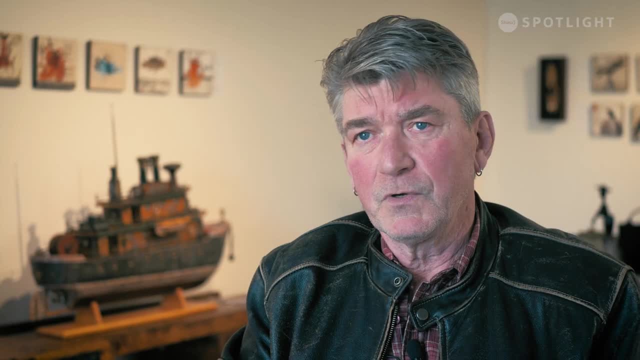 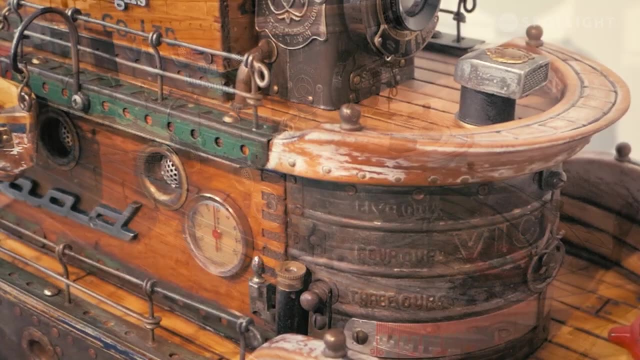 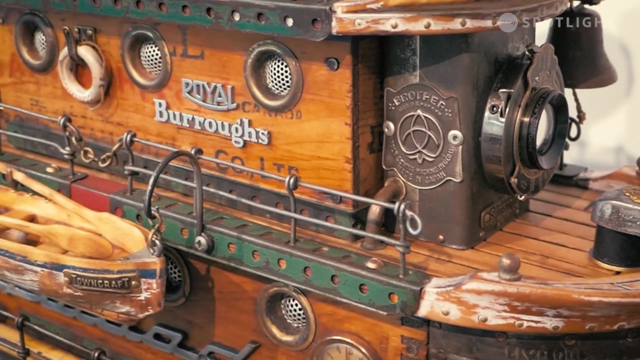 As I've grown and gotten more experience, I think my art now is better than it was. I think steampunk's brought me to a good place as far as my skill sets, being able to exercise them and put them all together. It just kind of works for me.